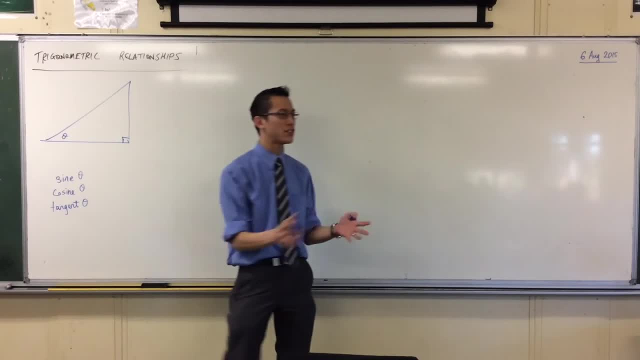 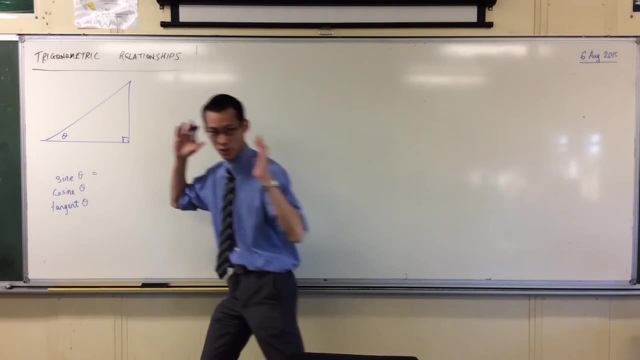 It tells you a relationship between these three angles. It tells you a relationship between some of the sides right. Help me out sine theta. what would it be equal to Like? what's that actual ratio? what's the ratio defined as? 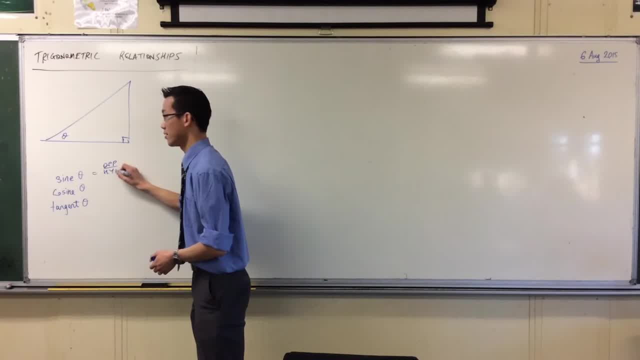 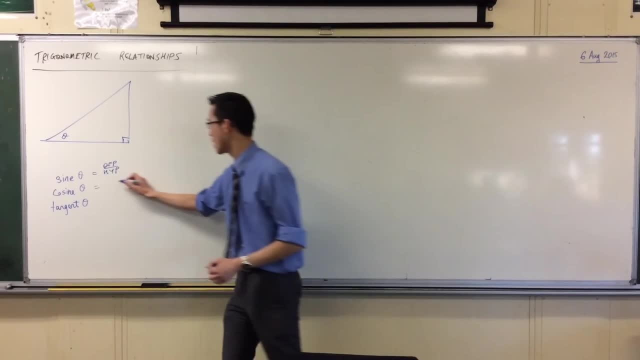 It's opposite on hypotenuse. very good, Opposite on hypotenuse. good morning Cosine cosine. think back to yourself, okay, Adjacent over hypotenuse, thank you. And then, of course, your last one, tan. you can think of two ways. 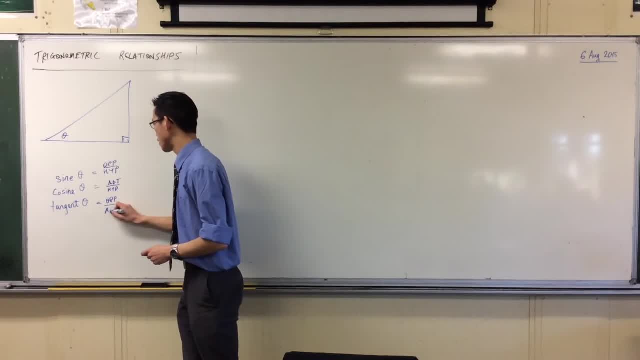 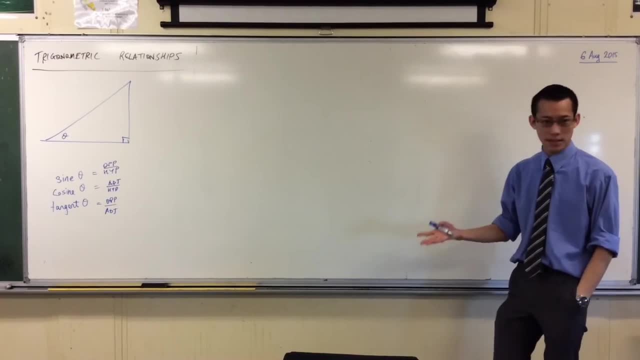 The first way you learn is you go opposite over adjacent Right, And so that's where you get soccer toe out of this right. But there's a second way which you may not have seen before, but if you have, it's okay. 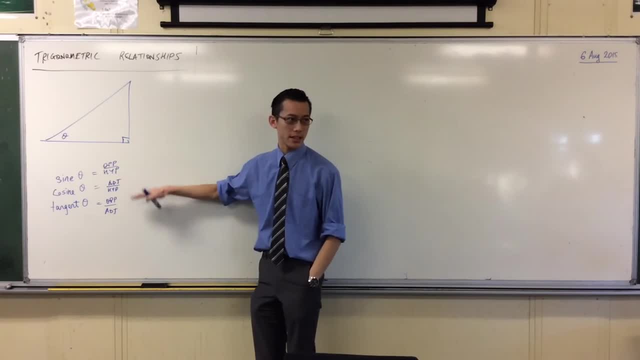 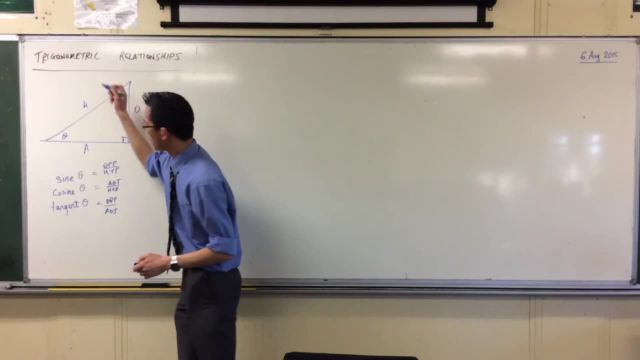 That's what we're going to be focusing on today. See how you've got these three things, these three quarters, and clearly they are all related to each other, right? You've got your opposite side here, your adjacent side here, your hypotenuse there, right? 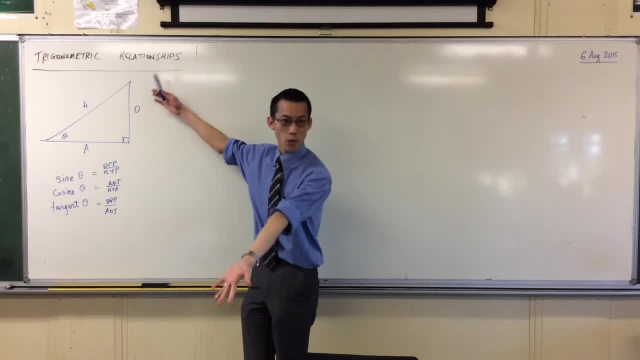 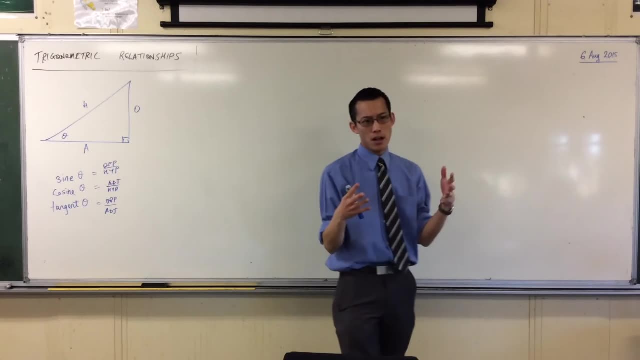 If I had some numbers on these, like say, your typical right angle triangle would be three, four, five, You're going to get three fifths, four fifths, three quarters. okay, These numbers, the exercises you get given, you just say, okay, work out what sine theta is. 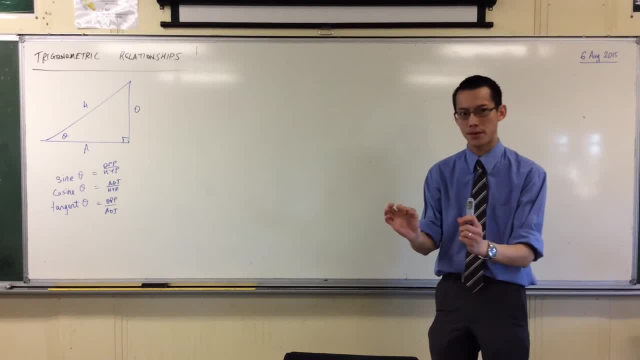 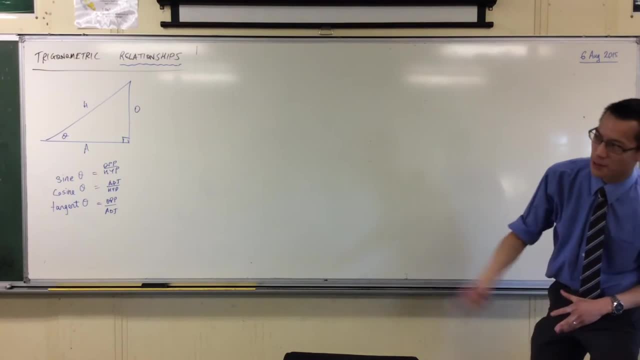 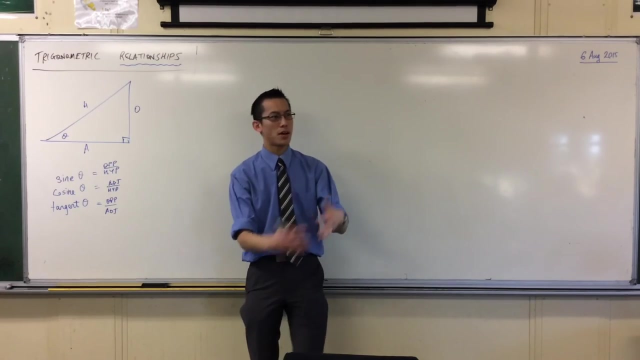 Work out what cos theta is, and on and on and on. And you're just working out numbers. But what doesn't get emphasized so much? come in, come in, grab a seat. What doesn't get emphasized so much is that these three things, they must be integrally linked. 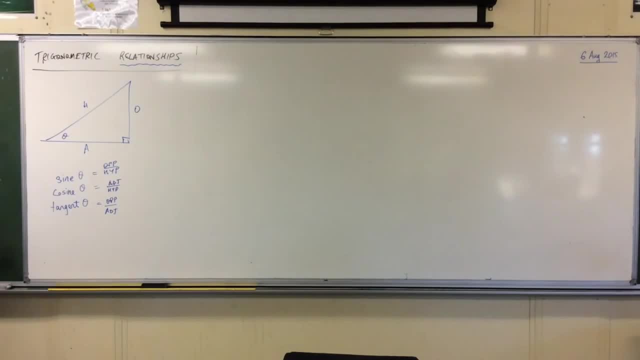 They have a relationship with each other. okay, Sorry, It's cool You can see, for instance, right, This is one of the less obvious things. But tan, right, Tan is not just the relationship between these two sides. Okay, if you just came in, get your things out, get what's down on the board. 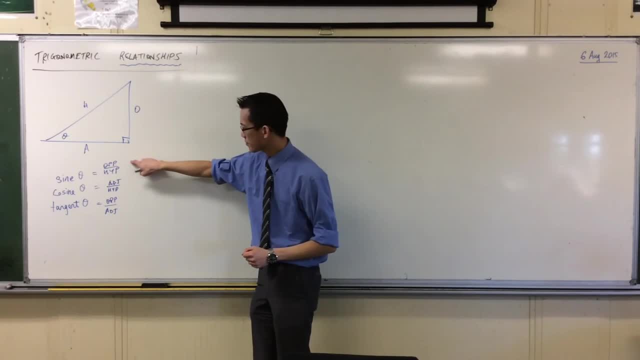 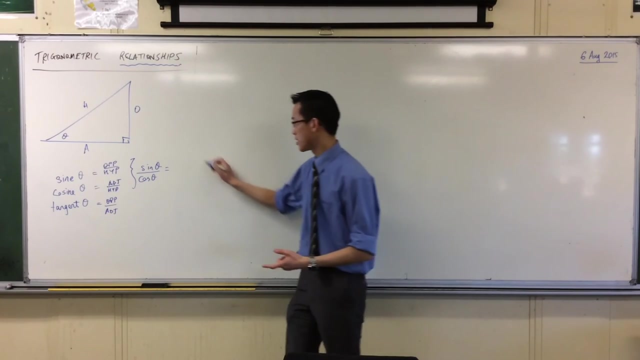 You can see if I take sine and divide it by cosine, right? Do you see this? See how they both have the same denominator, right? So if I did sine divided by cosine, I could just quickly write this up. This is going to be opposite. on hypotenuse divided by adjacent. on hypotenuse right.